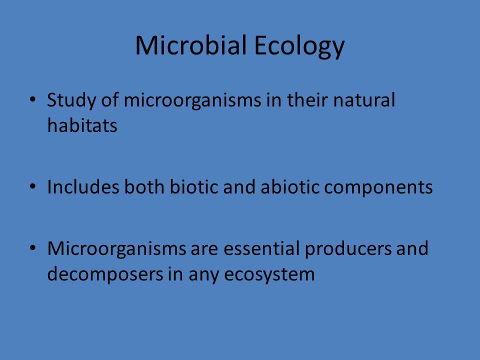 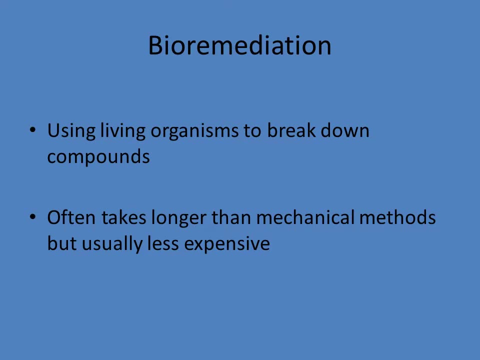 ecosystem. They're also decomposers. They play a very important role in nutrient cycling. Bioremediation is using living organisms to break down compounds. This is a large area of microbiology, of using both bacteria and or fungi to break down some of these. 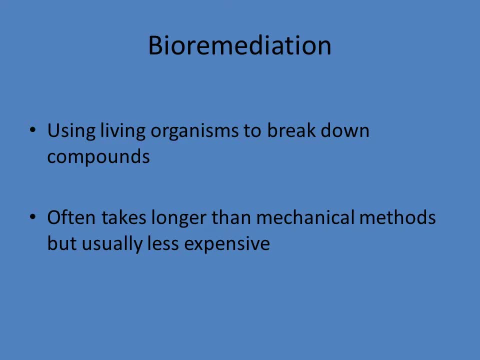 hazardous compounds that have accumulated, usually in the soil, Instead of using mechanical methods of cleaning up the soil, such as digging up the soil, taking it to an incinerator, burning off the hazardous materials. all that takes time. It takes a lot of money to do that. 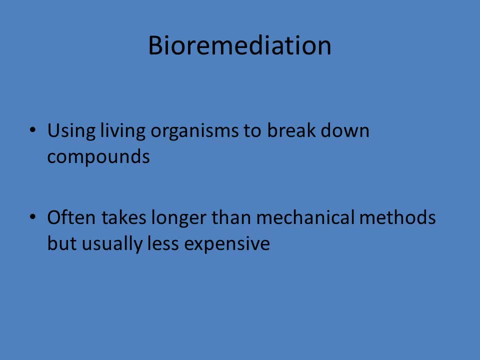 Instead of bioremediation, instead of removing that contaminated soil, it's bringing microorganisms that can break down the hazardous materials that are in it. Will it take longer? Yes, probably so, but it's going to be less expensive. You don't have to say. 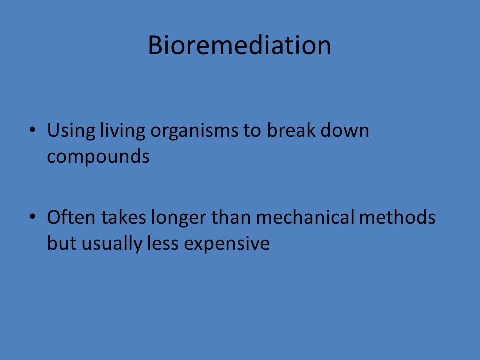 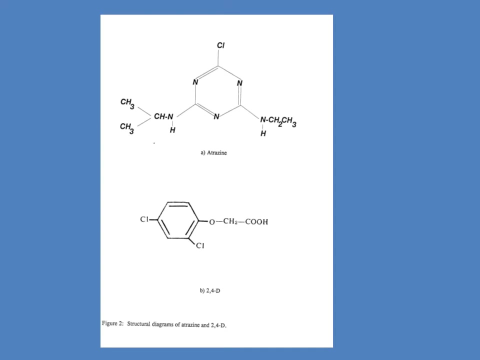 haul off the contaminated soil and then replace it with clean soil. You leave it be and you just bring the microorganisms that naturally exist in the soil anyway and have them basically clean. These are just some examples of things that can be done. This shows two different herbicides. 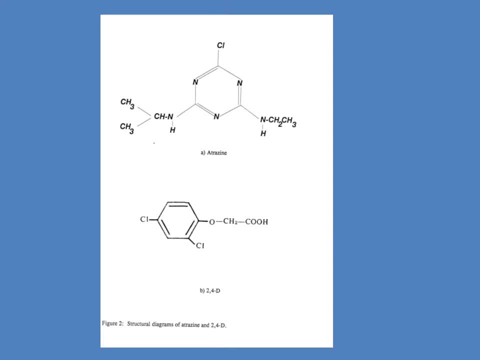 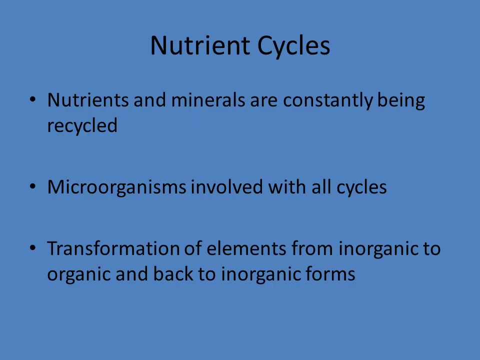 atrazine and 2,4-D. Because they have chlorine on it, it's a little bit harder for them to be broken down in nature. Those were some that I had looked at years ago in some of my research of microorganisms that were capable of breaking those down. 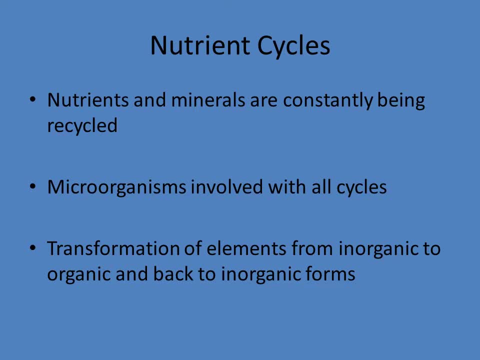 So I'm going to show you some of the things that can be done to clean up the site, And when I talk about breaking it down, I mean converting it to CO2 and water completely. Nutrient cycles: your nutrients, your nitrogen, your phosphorus, your sulfur. 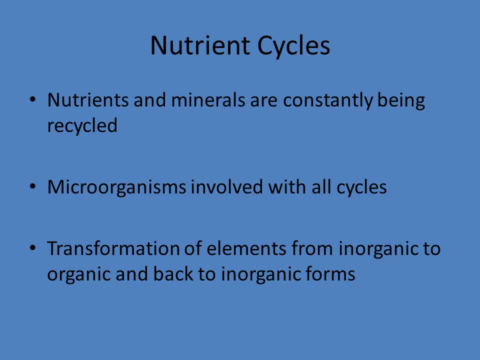 carbon. all of that is constantly being recycled. How does it get recycled? Well, microorganisms are going to be involved with that. They're going to transform those elements from inorganic to organic forms, and then back again, And this just shows an example of this. 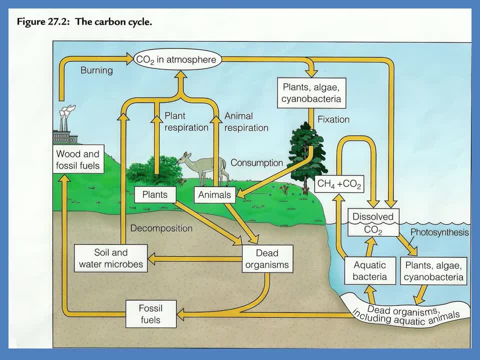 carbon cycle. As animals and plants die, the decomposition returns that carbon back into the soil. Microorganisms that are found in the soil will often then break it down further, releasing some of the CO2 into the atmosphere Over long, long stream periods of time. 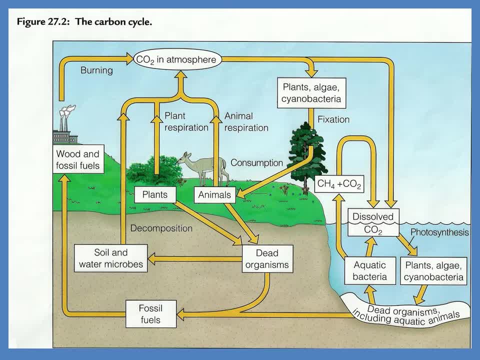 dead animals will help form fossil fuels which then we recover That's burned, putting CO2 in the atmosphere. Plants, algae, cyanobacteria take up through photosynthesis that carbon dioxide and form it into sugars like glucose et cetera. that then animals will eat And then, as animals, 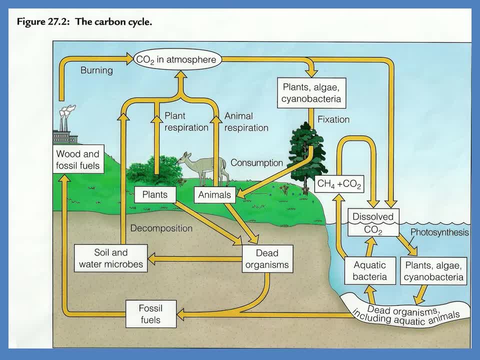 die. there it enters back into the cycle again. Some of the CO2 is dissolved into oceans and is used by aquatic bacteria. It's used by algae, cyanobacteria, et cetera. So it just gives you an idea of how everything gets recycled. 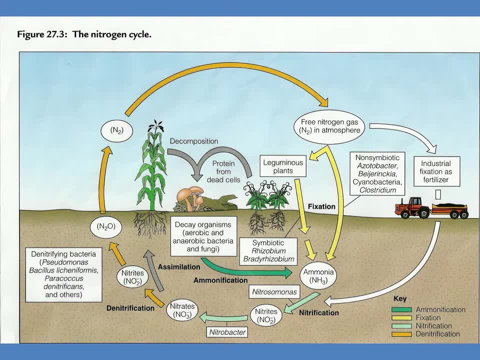 And it's not just carbon, It's also things such as nitrogen, And microorganisms are very critical players in the nitrogen cycle, because sometimes nitrogen is in the soil and it's in a form that, say, plants cannot use, And so it's the bacteria. 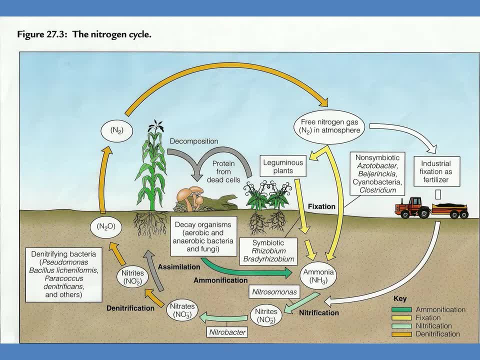 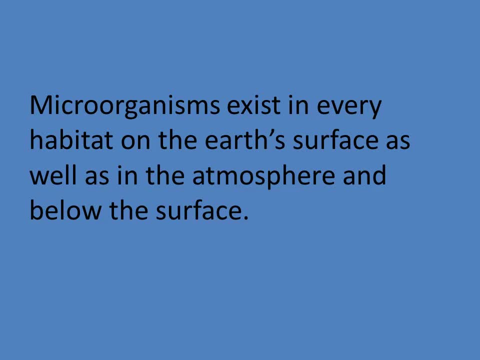 it's the fungi that convert it into a form that then can be used. So we've found the microorganisms. It's a very important one. So we've found the microorganisms. microorganisms, they're everywhere. they're below the surface, deep subsurface, in the ocean. 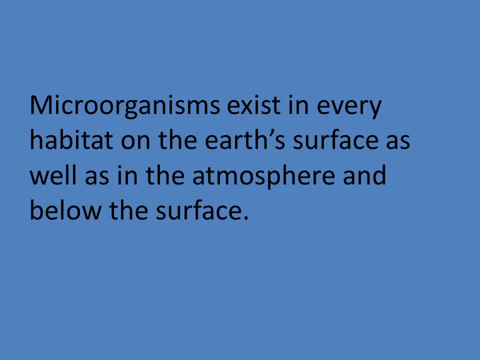 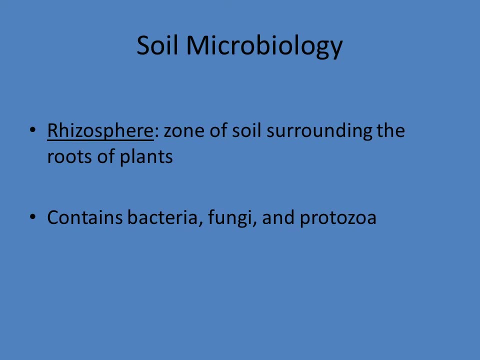 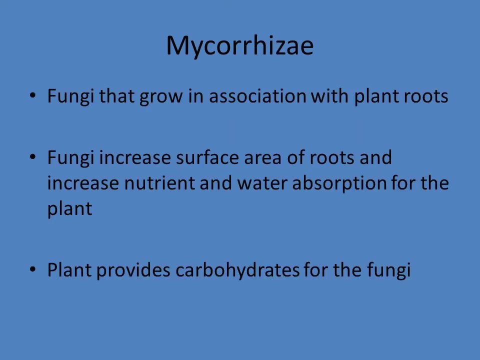 they're up at high in the atmosphere and everywhere in between soil. microbiology: this is another specialty area. the soil is going to contain bacteria, fungi, protozoans and sometimes people specialize. looking just at the rhizosphere, this is the area, the soil that's surrounding the roots of plants. this is a very active area of living organisms. one type of 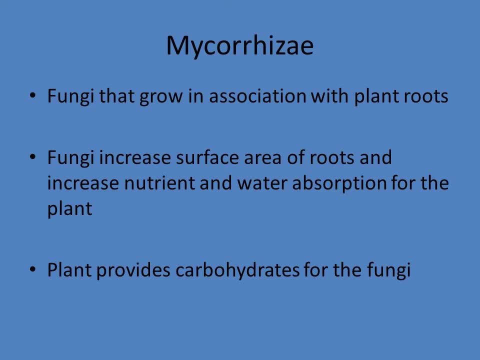 fungi that grows there are known as the mycorrhizae. these are fungi that do grow in association with plant roots. over 80% of your plants must have mycorrhizal fungi associated with them to have good growth. why are the fungi there? well, it's a symbiotic relationship. the fungi, 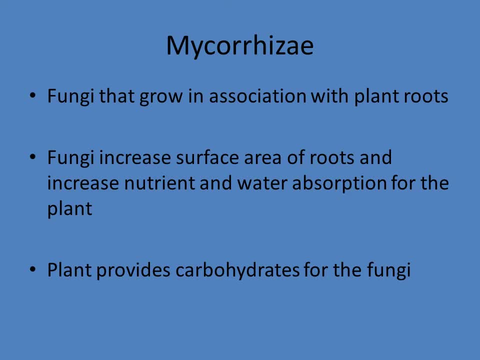 are the ones that grow the most in the soil. they're the ones that grow the most in the soil. fungi are going to help increase the area, the surface area of the roots that it can expand out into the soil, to absorb nutrients, to absorb water the plant is providing through photosynthesis. 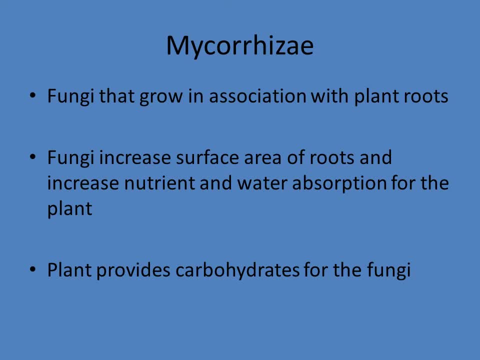 carbohydrates for the fungus fungi to grow, so the fungus is benefiting from the sugars from the plant, the plant is benefiting from the nutrients and water absorption by the fungi, and the fungi actually also provide some protection because it will be covering the plant roots in some cases. one thing that we have seen is that 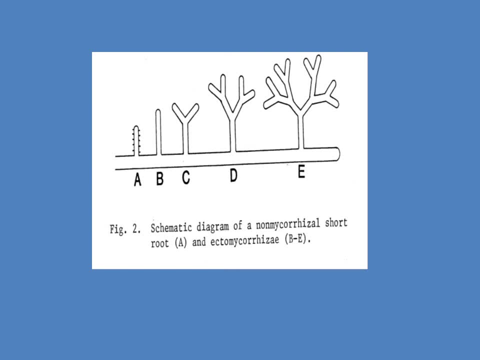 when you have a plant root on this example, as you see on a- would be without any mycorrhizal fungus associated with it. when it is infected with a type of mycorrhizal known as ectomycorrhizal, you tend to have this. 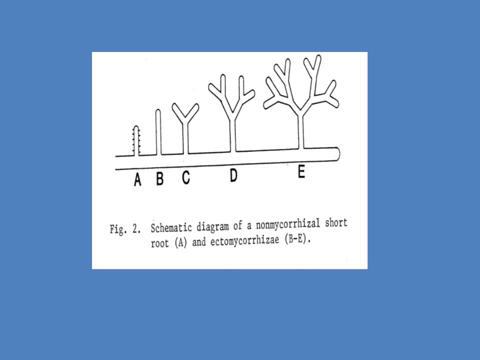 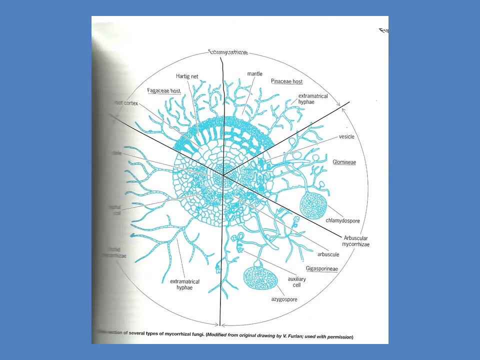 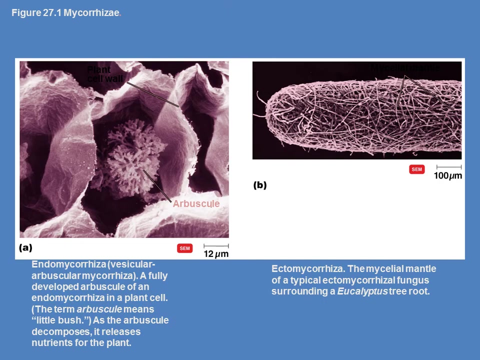 increase branching of the roots, once again increase surface area. that's only going to benefit the plant. and this is just showing a slide showing how all different types of fungi can infect the roots and cause different structural changes within the roots, some more dramatic than others. on the picture on a 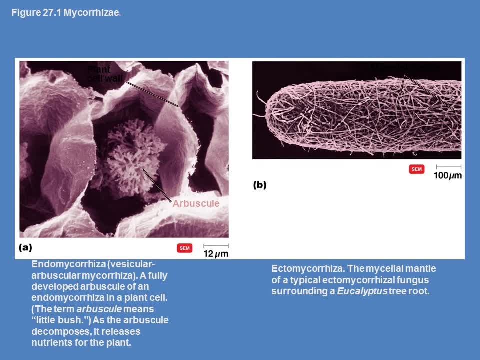 that is what we call endomycorrhizal fungi. that is what we call endomycorrhizal fungi. that is what we call endomycorrhizal fungi are known as also known as a VA or Vesticular, ovascular mycorrhizal, and that 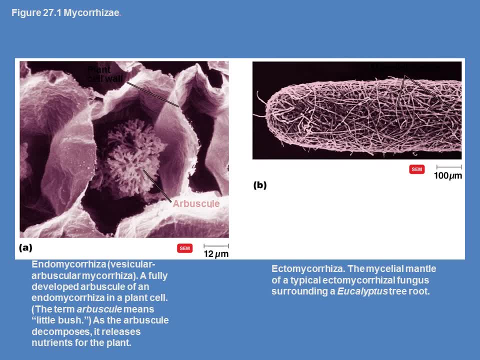 is what it is going to. that is, the fungus that is actually inside the cell of a plant root B, actin mycorrhizal and in this case, the mycelium, the long strands, individual strands, hyphae and right. it completely covers the root. this 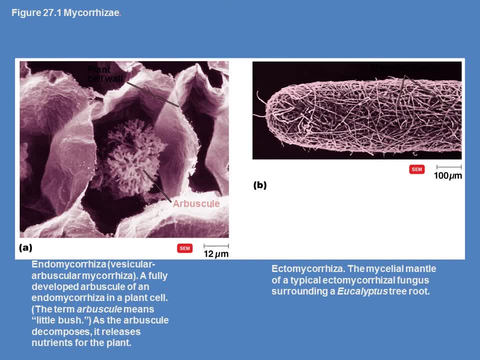 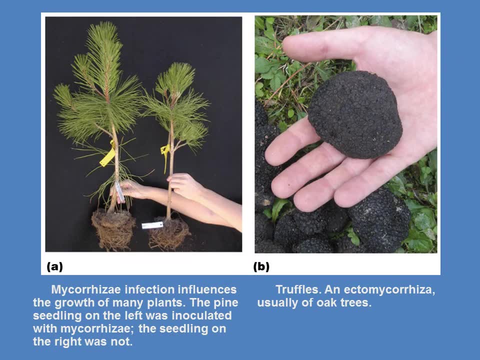 is like putting a coat around the kleenex, then you wrap it all over with root protecting it. so anything that is absorbed is going to go through the fungus first. so the overall effects of having the mycorrhizal fungi once again in A. as you can see, these are pine seedlings. the one on the left has.